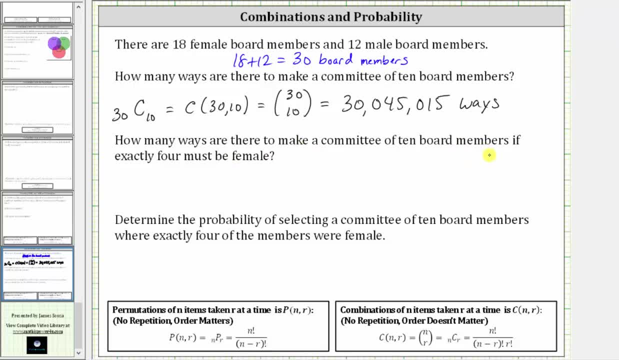 that means exactly six must be male, which means to determine the number of ways to make a committee of 10 board members if exactly four must be female. you must determine two things: the number of ways to select exactly four females and the number of ways to select exactly six males. 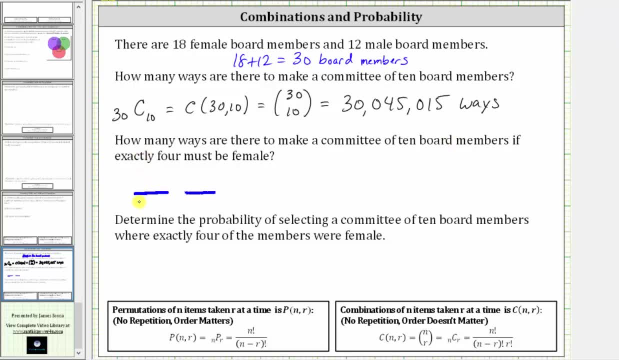 to make a committee of 10.. So this will look like this. So this will be the number of ways to select four females. This will be the number of ways to select six males, And because there are 18 females and the order doesn't matter, 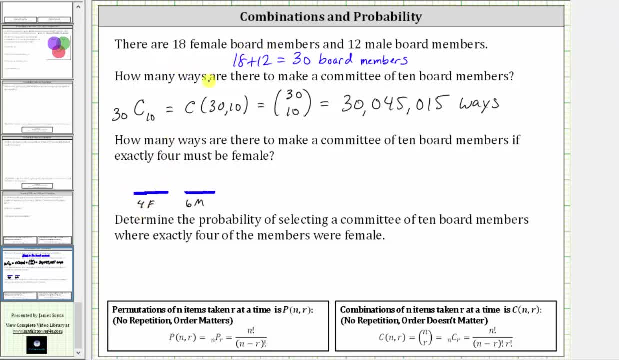 the number of ways of selecting four females from 18 females is 18- choose four again, because order doesn't matter. And then we have times the number of ways of selecting six males from the 12 male board members, which is 12- choose six. 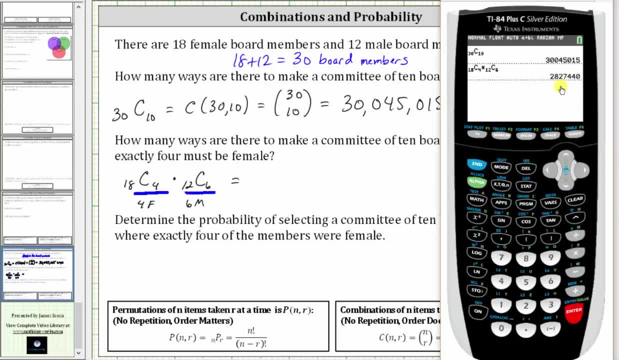 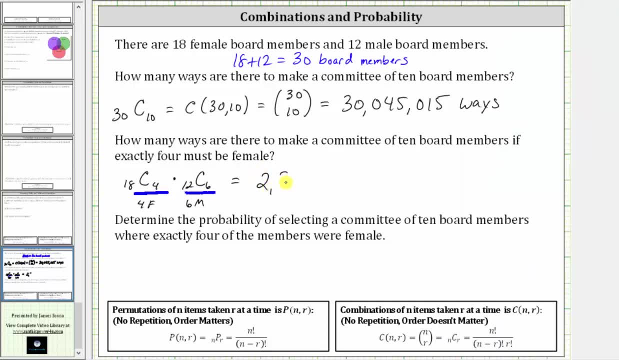 And now to determine this product on the TI-84, which is 2,827,440,, which means there are 2,827,440 ways to make a committee of 10 board members if exactly four must be female, which also means exactly six must be male. 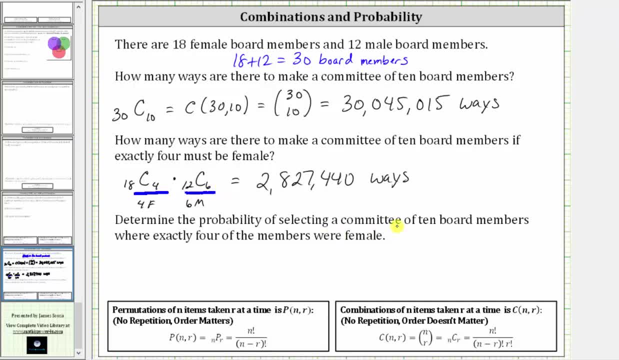 And for the last question, we're asked to determine the probability of selecting a committee of 10 board members where exactly four of the members were female, which again also means exactly six of the members were male. So we'll say the probability of exactly four females. 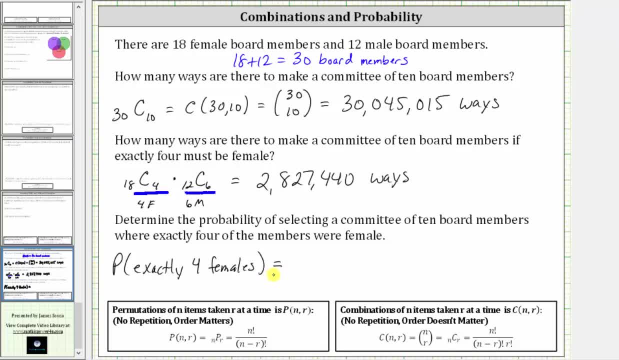 and we know this is equal to the favorable number of outcomes divided by the total number of outcomes, And the favorable number of outcomes and the favorable number of outcomes is the number of ways to make a committee of 10 board members, if exactly four must be female. 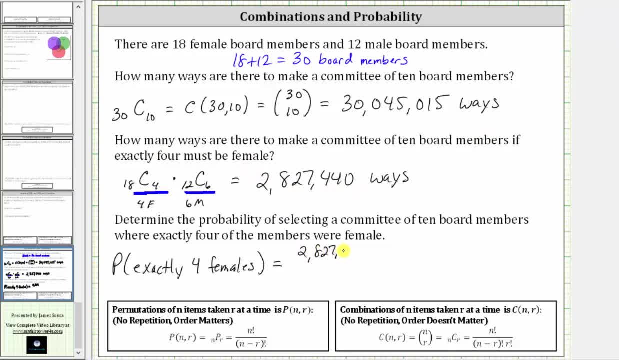 which is 2,827,440, divided by the total possible number of outcomes, which is the number of ways to make a committee of 10 board members from all 30 members, which is 30,045,015.. Let's go ahead and find this quotient. 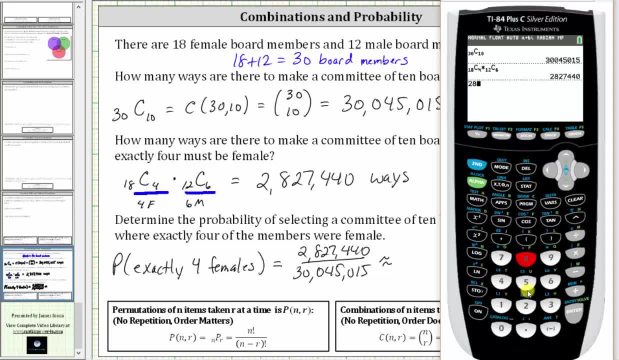 Let's go ahead and find this quotient: Again: 2,827,440 divided by 30,045,015,. Again 2,827,440 divided by 30,045,015,. Again 2,827,440 divided by 30,045,015,.